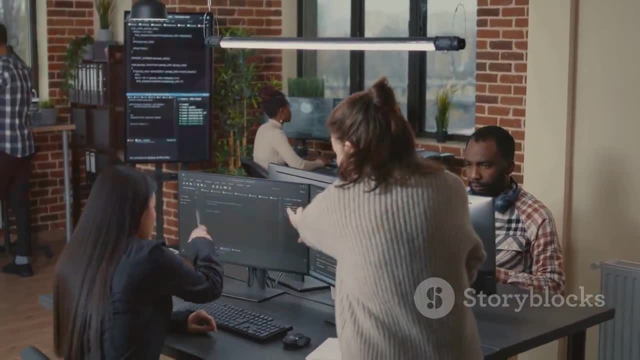 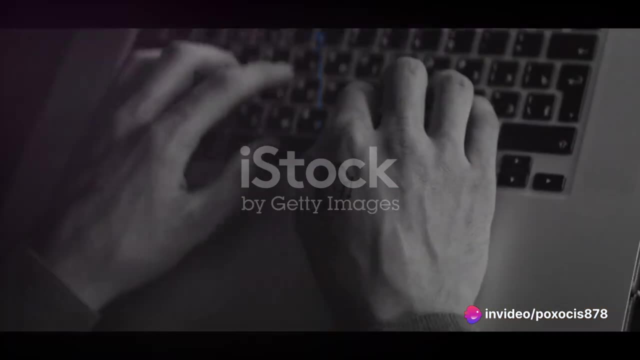 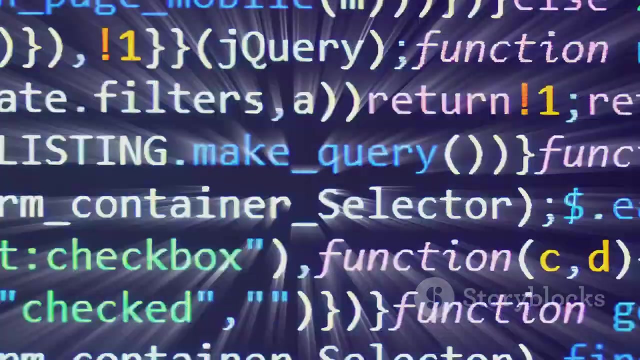 It's like a seasoned mentor, guiding you through every step of the journey, ensuring that you not only learn Prolog but also understand its nuances. So why wait? Embark on a journey of discovery and innovation. Experience the power and potential of logic programming with Prolog. 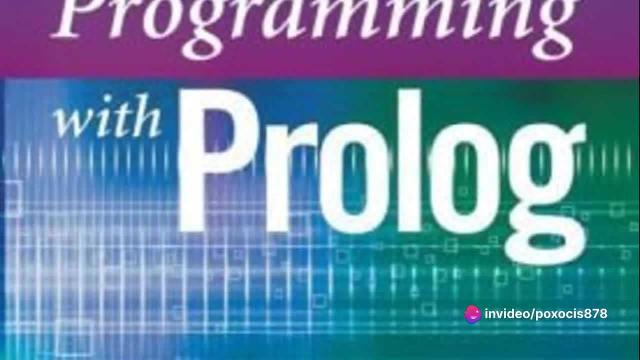 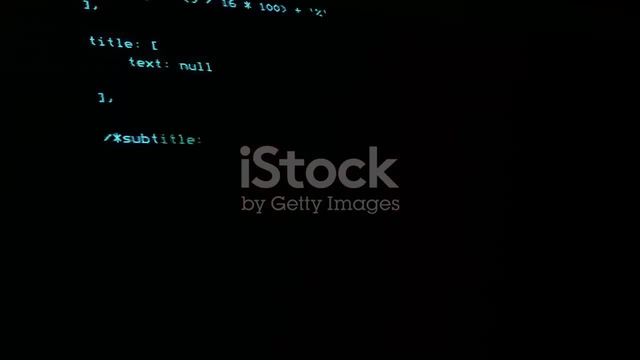 Purchase the ebook today and open the door to a world of endless possibilities. The world of Prolog awaits you. Your journey into the future of programming starts now. Don't miss this chance. Secure your ebook at an exclusive discounted price by clicking the buy button now. 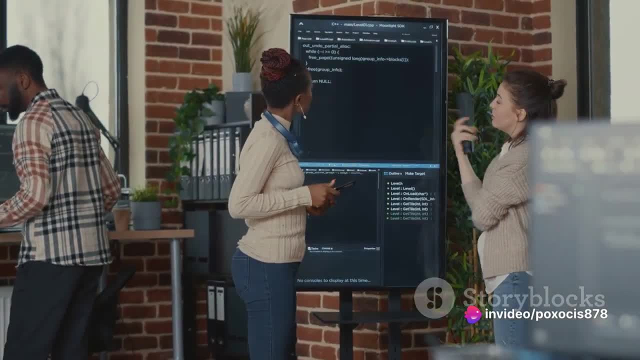 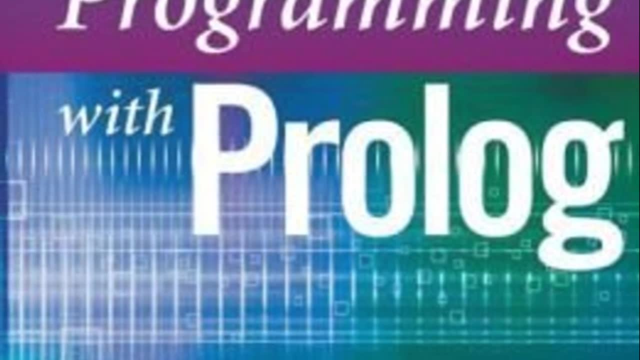 Dive into logic programming with Prolog And begin your exploration of the world of Prolog. The world of Prolog, The world of logic programming, The power of Prolog and the future of programming are within your reach. Don't wait: Start your journey into the world of logic programming now. 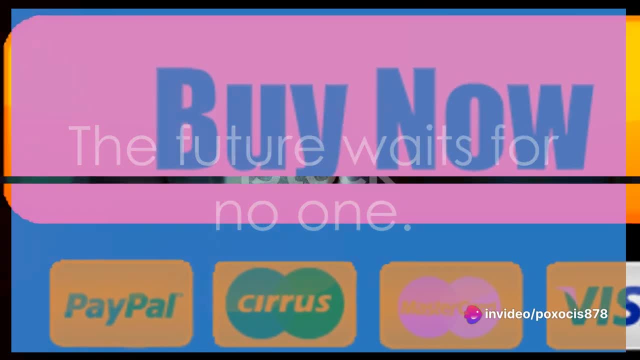 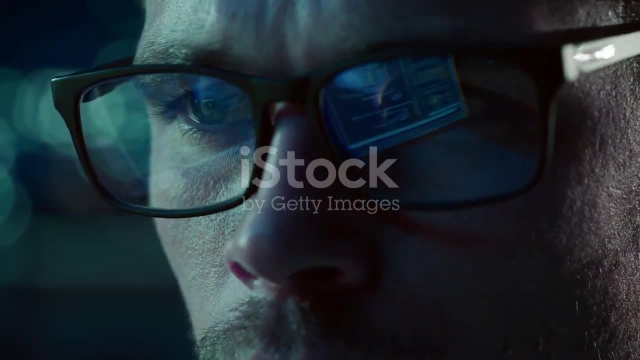 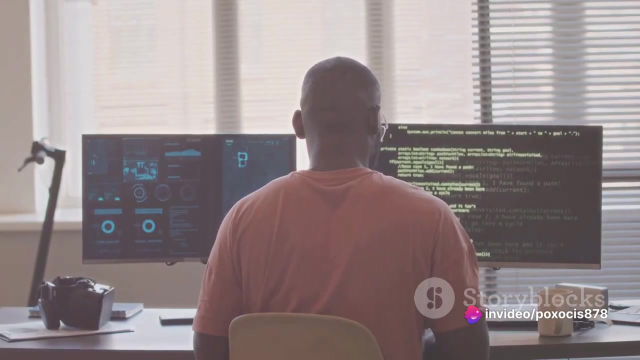 Remember: the future waits for no one. Make your move. Grab your ebook now. John Smith, software developer. Logic programming with Prolog is a superb ebook that has aided me in my exploration of the field. Prolog is understandable to newcomers like myself because of the writer's clear and simple. 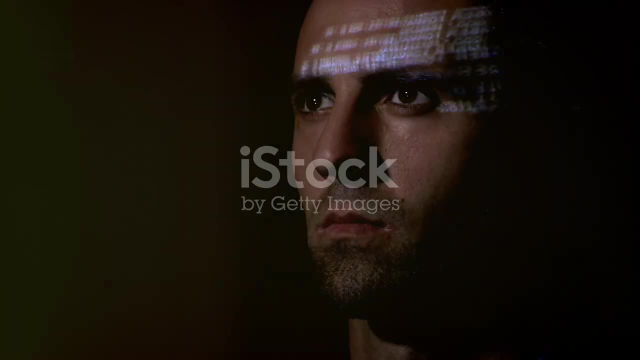 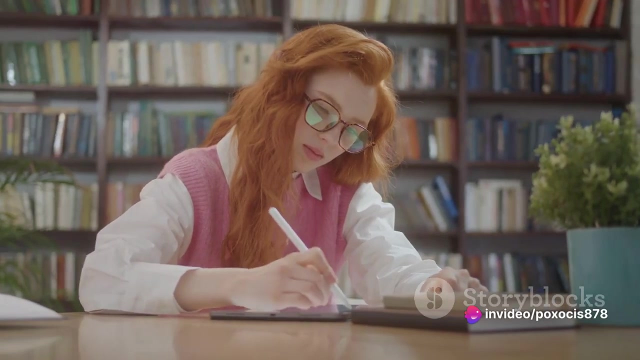 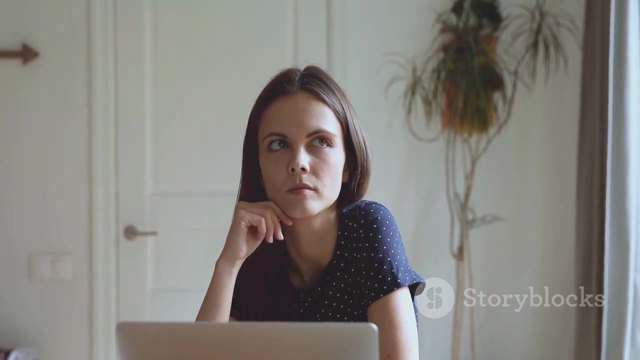 understanding of its core ideas. With the help of the ebook's many examples and exercises, I was able to strengthen and practice my comprehension of Prolog's logic-based programming paradigm. Sarah Thompson, computer science student, Logic programming with Prolog ebook surpassed my expectations. 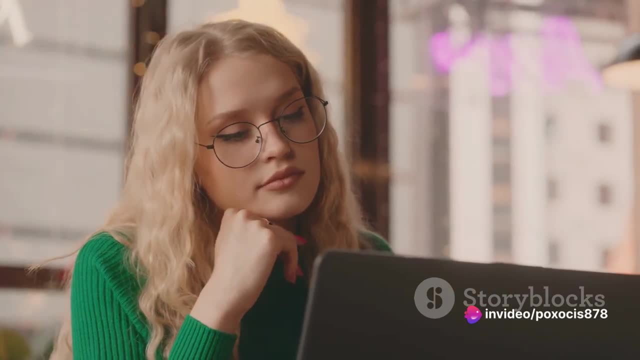 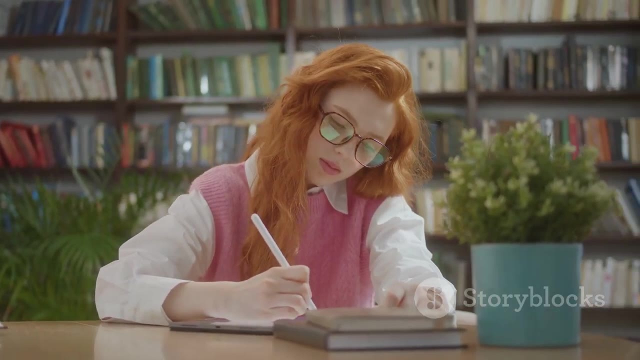 I had been looking for a thorough resource to learn Prolog. The ebook offers a strong grounding in the concepts and methods of logic programming. The portions on list manipulation and recursive programming were my favorites because they gave me a thorough understanding of Prolog's possibilities. 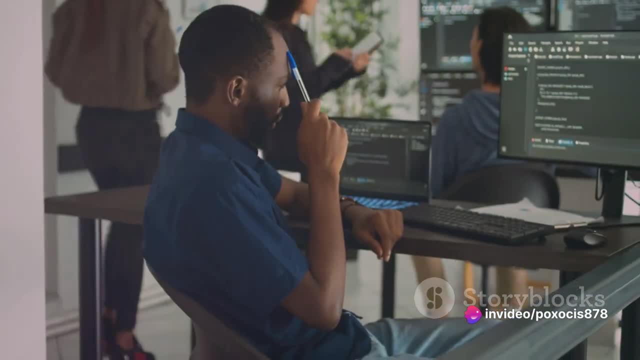 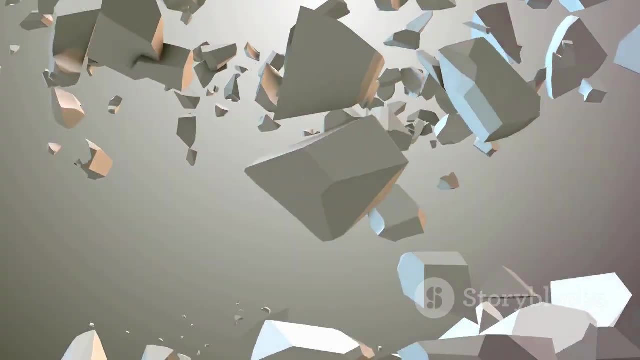 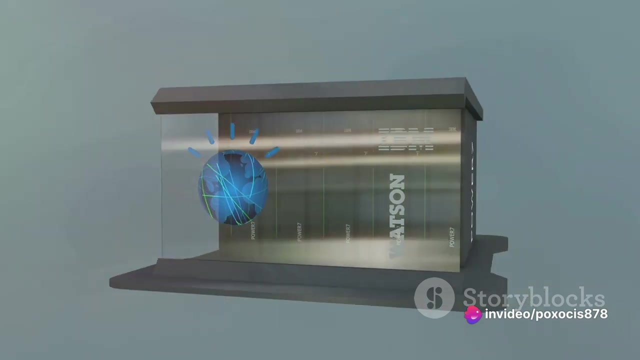 Michael Johnson AI researcher. The subjects covered in the ebook range from fundamentals of Prolog to more complex ideas like constraint logic programming. The authors also discuss practical uses of Prolog, such as expert systems and natural language processing. The well-organized and thorough logic programming with Prolog ebook is a resource that will 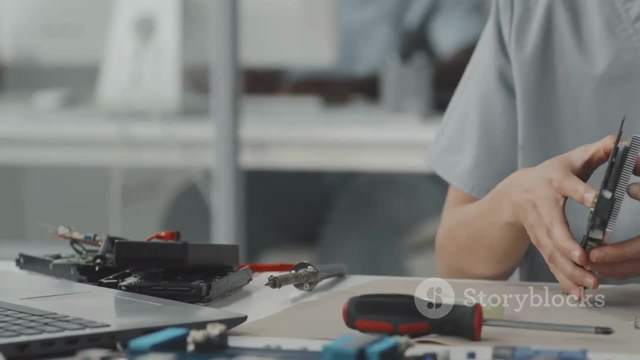 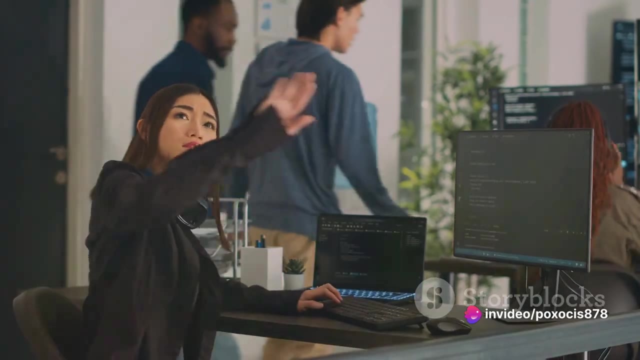 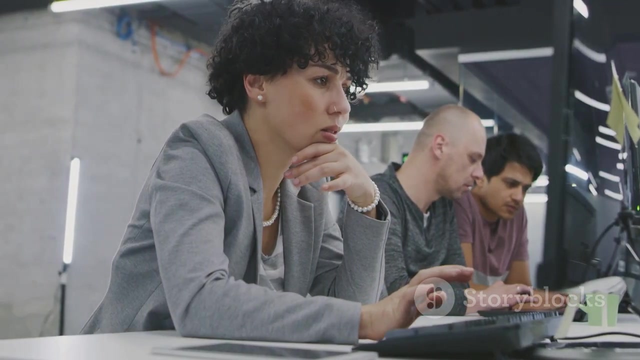 be useful to programmers of all levels. Sarah Thompson, software engineer. As a software engineer, I found the Logic Programming with Prolog ebook, which I purchased, indispensable. It comprehensively covers all essential concepts of logic programming using Prolog, thus making